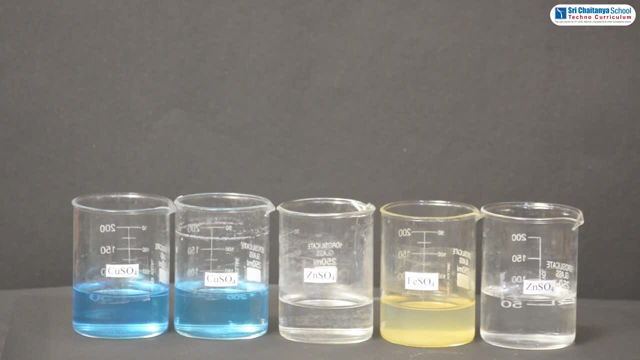 Take 5 beakers and add small amount of water in each beaker and dissolve copper sulfate, zinc sulfate, iron sulfate in the different beakers And arrange all beakers in an order by following: copper sulfate in the first beaker, again copper sulfate in the second beaker. 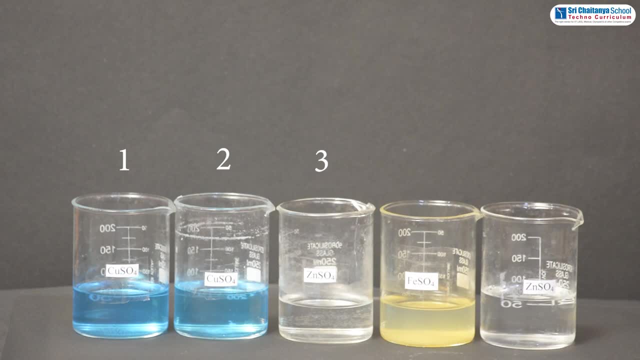 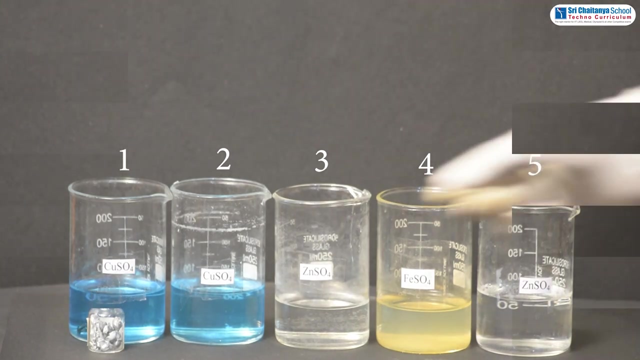 zinc sulfate solution in the third beaker, iron sulfate solution in the fourth beaker and finally, zinc sulfate solution in the fifth beaker. Now add zinc granules to leftover minerals. first beaker which contains copper sulfage. In a similar way, add iron nails to the second beaker. 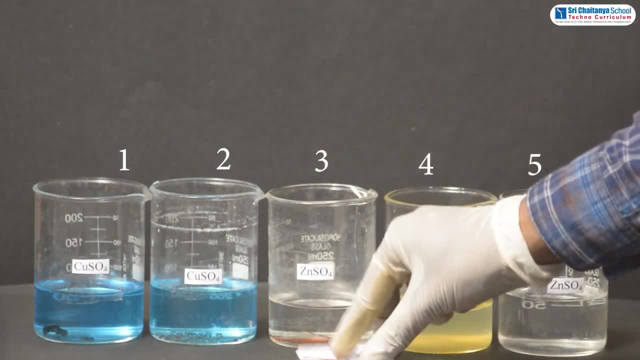 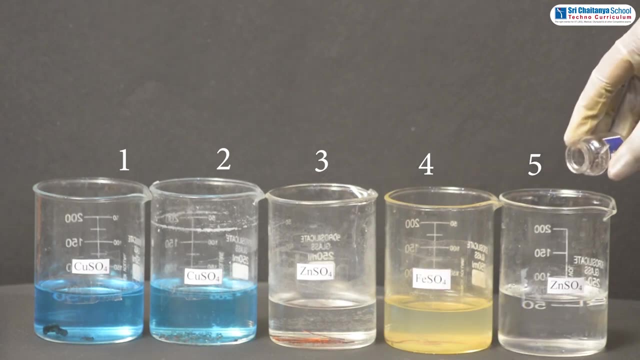 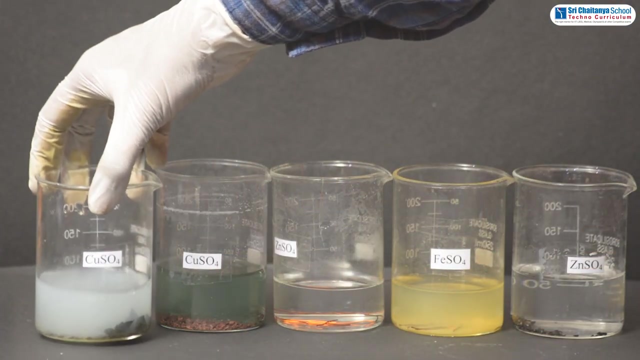 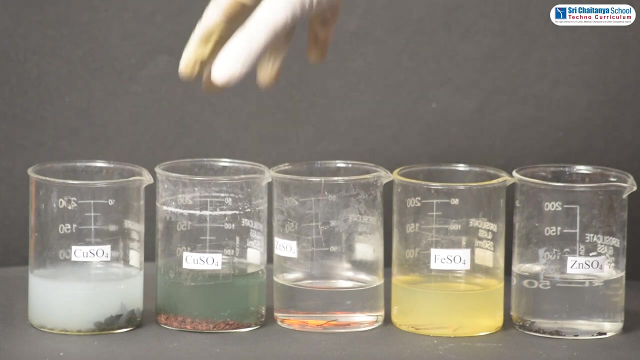 Add copper tunnings to the third and fourth beakers and again add iron fillings to the last beaker. Observation: In the first beaker, zinc displaces copper from copper sulfate, giving rise to a colorless zinc sulfate solution. Iron displaces copper from copper sulfate in the second beaker, leaving. 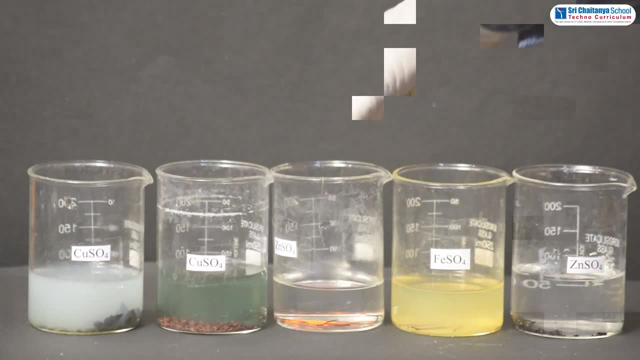 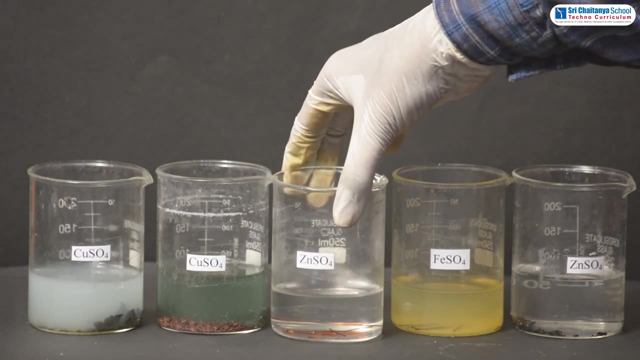 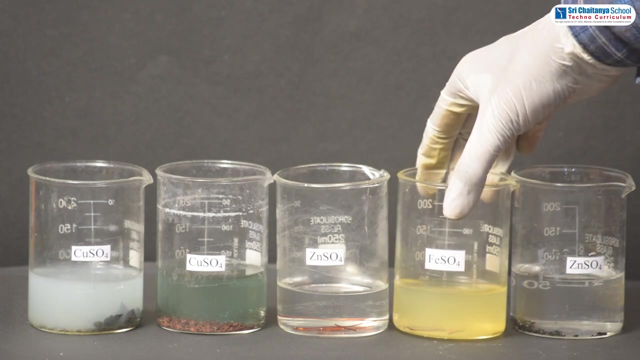 light green color of iron sulfate. And in third beaker, as we have added copper tunnings to the zinc sulfate solution, we cannot observe any change in that beaker as copper is less reactive than zinc. In a similar way in the fourth and fifth beakers also. 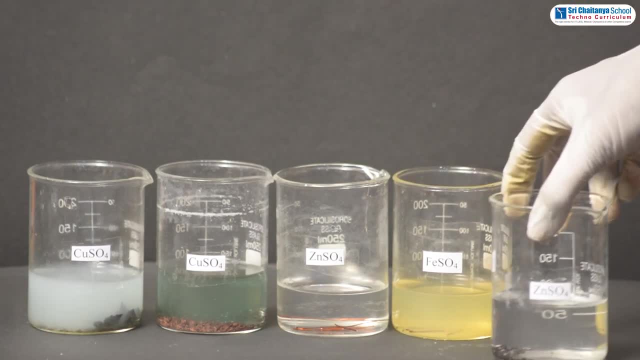 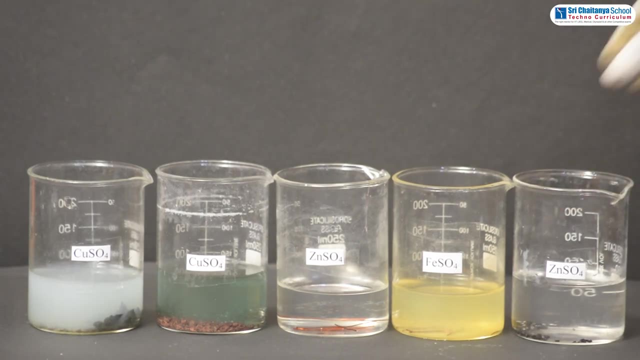 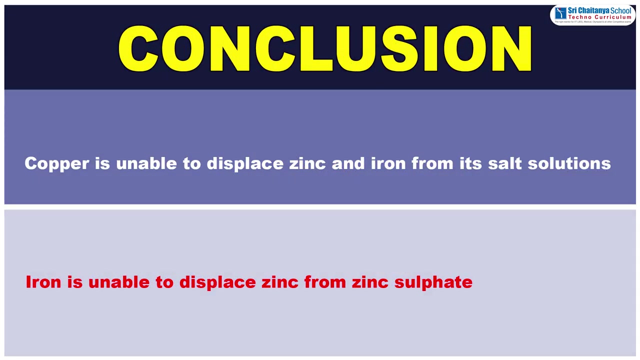 we cannot observe any reaction as these metals are less reactive comparing with the aqueous metallic salt solutions we have taken, That is, zinc sulfate in the last fifth beaker, iron sulfate in fourth beaker and again zinc sulfate in the third beaker. So finally, we can conclude that copper is unable to displace zinc and iron from its salt solutions.